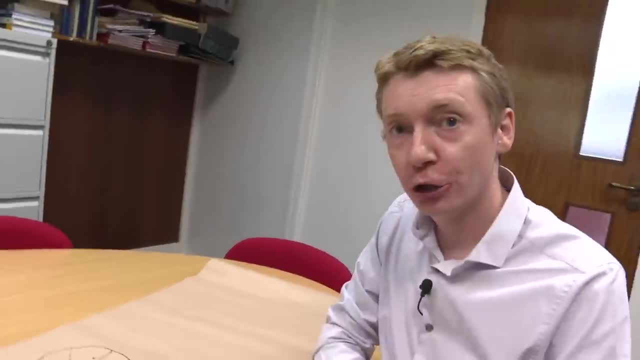 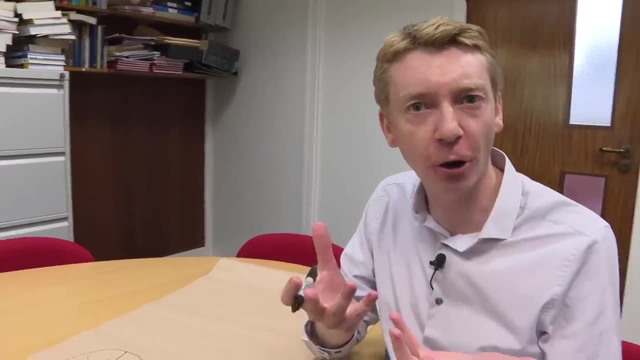 the question in the goat problem is: how long should the rope be if you want the goat to graze in half the field, and That feels like something you might be able to solve. Maybe with school level maths. you can get quite far with school level maths. Let's see how far we can get. 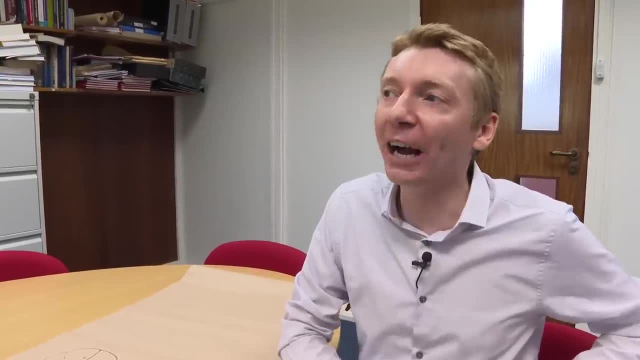 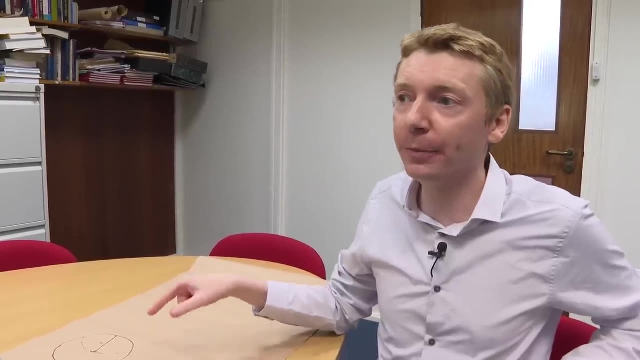 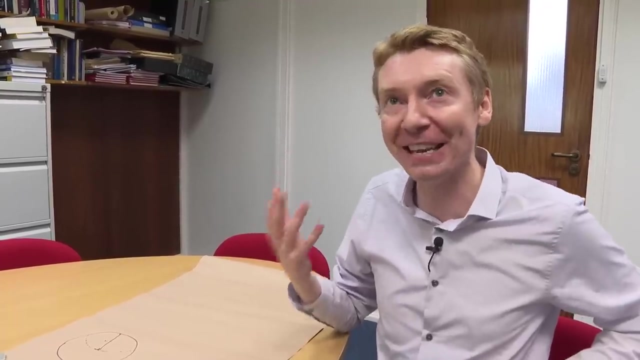 It feels easy. Yeah, it feels easy, And this is why people are so frustrated When you tell them this problem. I tell you what I gather: This is a problem that they used to teach a lot in US Navy academies. I don't know if they're teaching this as an example of being used to difficult problems, because they would teach this in these Navy. 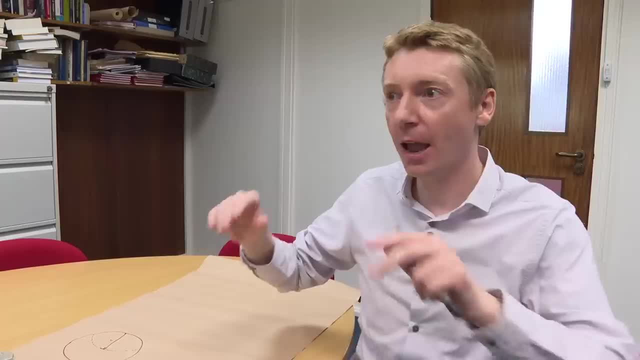 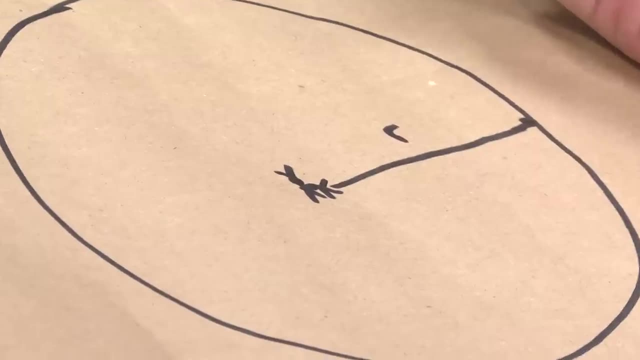 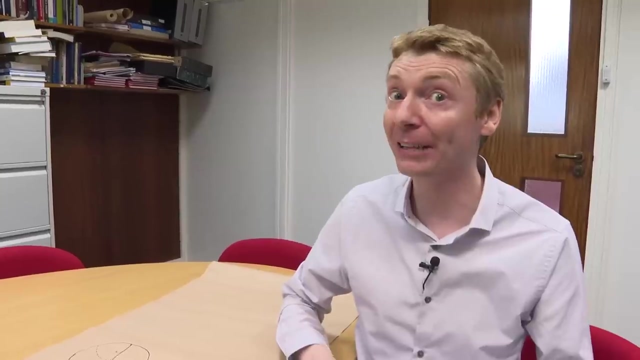 academies and they would say: and you can do this. there's no exact answer and people were frustrated and get surely This must have a exact answer. but no exact answer was found Until recently and it involves some hard maths. How would a school student attack this problem? 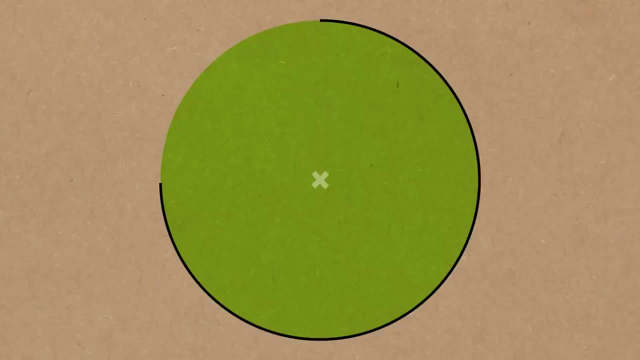 So let's do another circle, Let's make that the center of the field, do a little X for the center of the field and let's say My goat can eat some sort of circular area Like this, something like that, So my goat can reach all the way to the fence here and my goat could reach all the way to the fence. 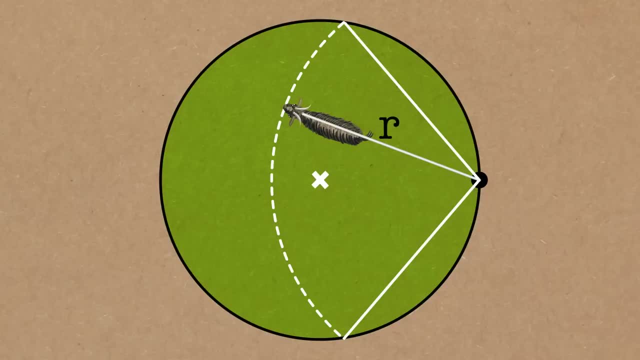 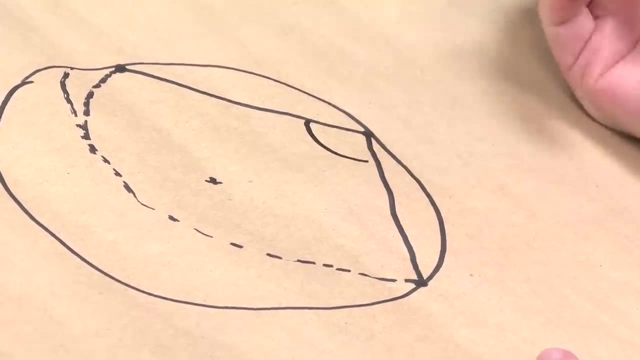 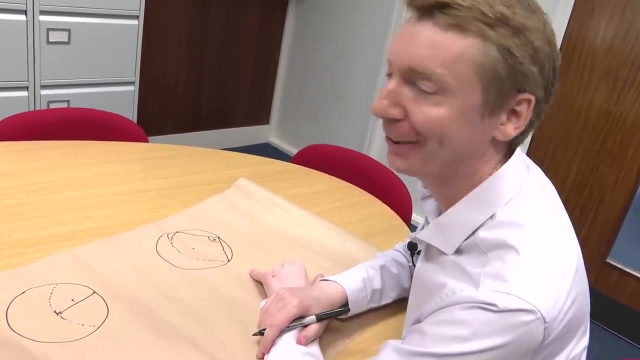 Here, and then he can eat all this kind of curve here. So it's a fraction of a circle with a radius of R, this angle here I've just made. let's give it a name Alpha. I'll use alpha for the angle. Why not? Okay, so good, It's a good name for now for an angle. good, grassy number. 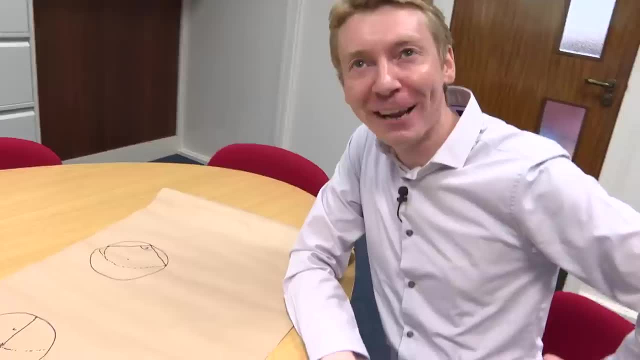 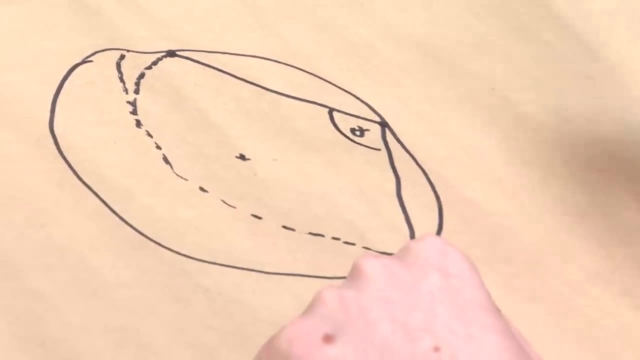 It's grassy alpha alfalfa. You think alfos, grassy alfalfa? Yeah, like I don't know. So this is how the you would start to calculate this with a bit of trig. I'm not going to go through all the details of the trig because it's boring. So what is the area of the field? 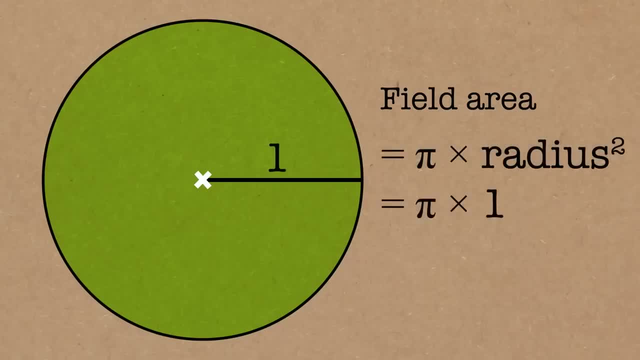 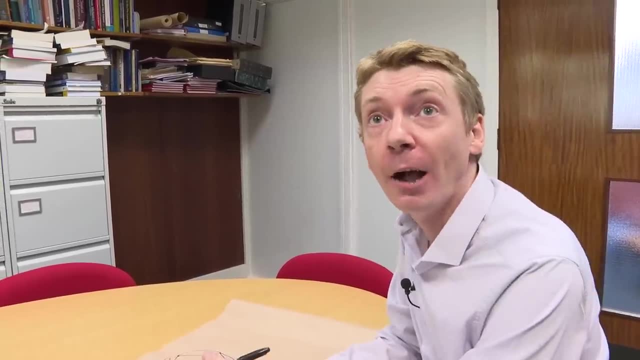 Well, it's a circular field. It has a radius of 1, so you use your traditional formula for working out the area of a circle and the field is going to Have an area of pi. But we want the goat to eat half the field, So pi over 2. 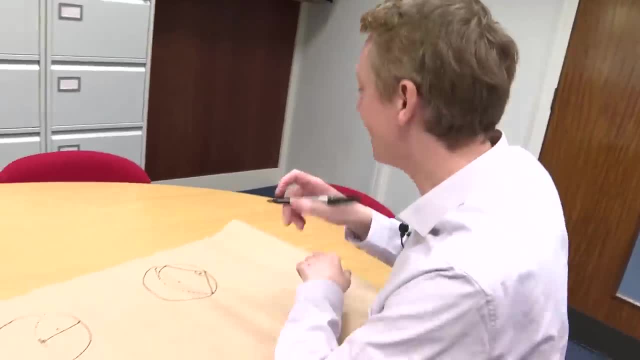 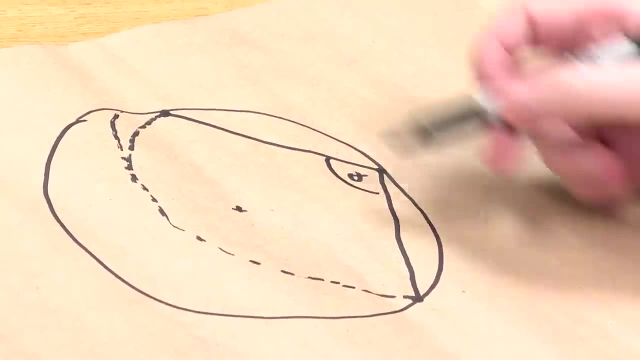 How about that? Okay, Pi over 2 is what the goat, we want the goat to have. Yeah, exactly, All right. Now you've given us his eating. Yeah, well, some of his eating area there. Yeah, so this is some of his eating area, isn't it? I've kind of missed off some bits here. I'll come to that as well. 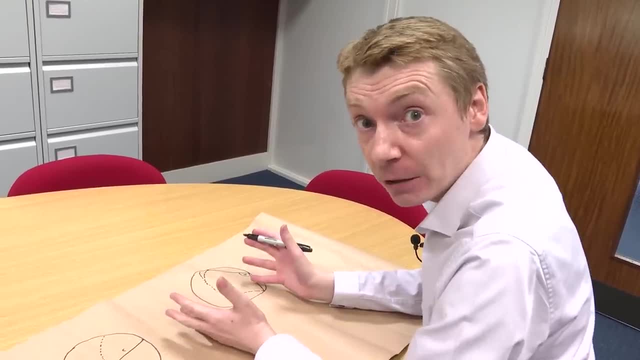 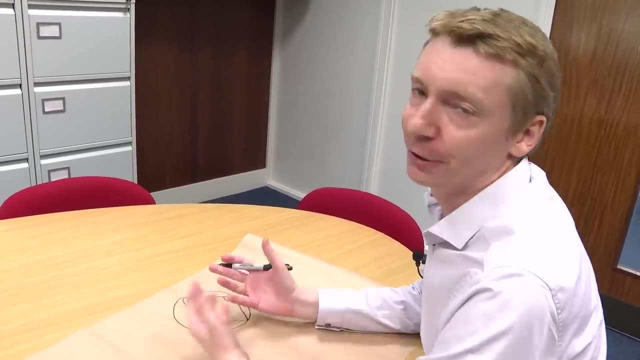 So what I'm going to do is a little bit of school-level trig. so when I say trig, I mean you know it's angles and signs and causes and Triangles and things like that. The length of the rope is going to be. 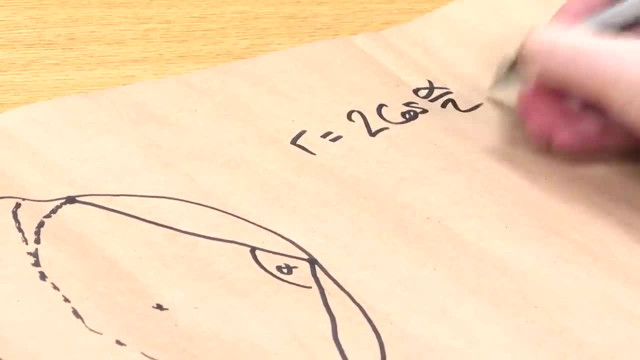 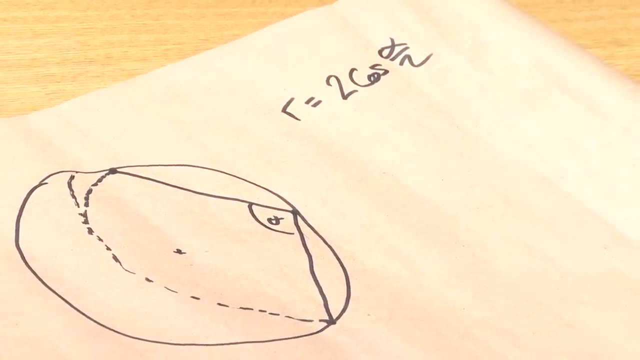 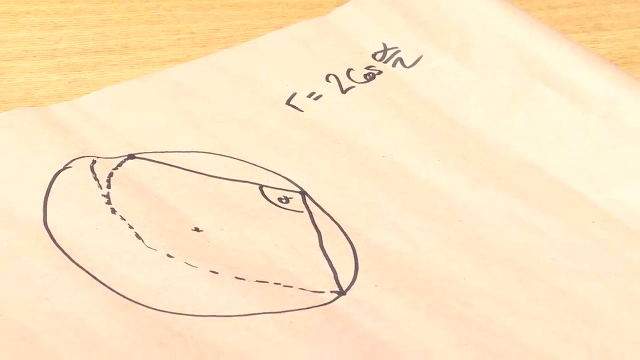 2 cos 2, And then it's alpha over 2.. It's half of this angle here, But it kind of doesn't help me work out the length of the rope. That's what I'm trying to work out, because now I've just Sort of changed the problem, because I need to work out what the angle is. Okay, so that's what we're doing next. 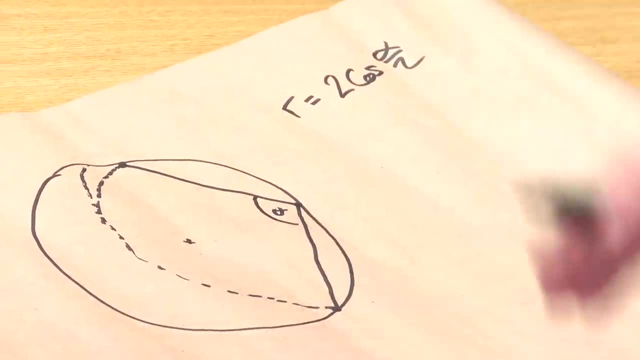 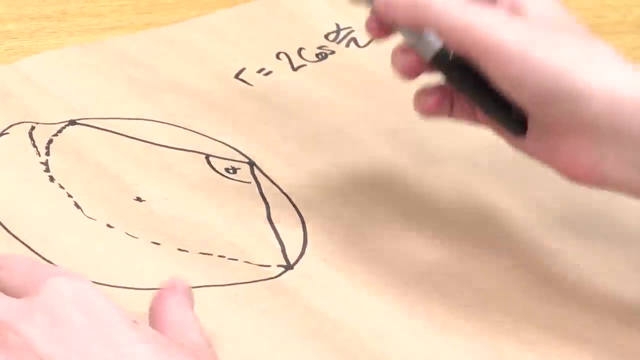 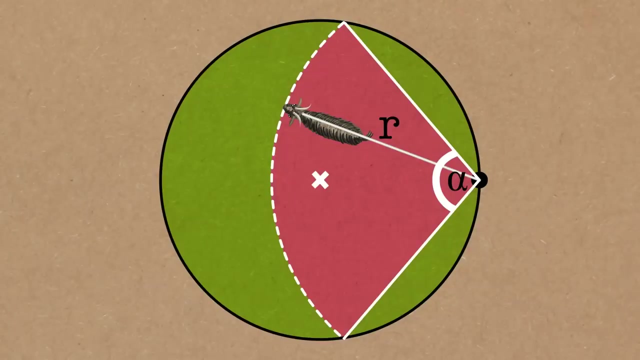 So that part is not so hard Working out. the angle is where it starts to get hard. Okay, so if you calculate this, what we can calculate is: Alpha is a fraction of a full circle, So I know that this area here is a fraction of a full circle of radius r. 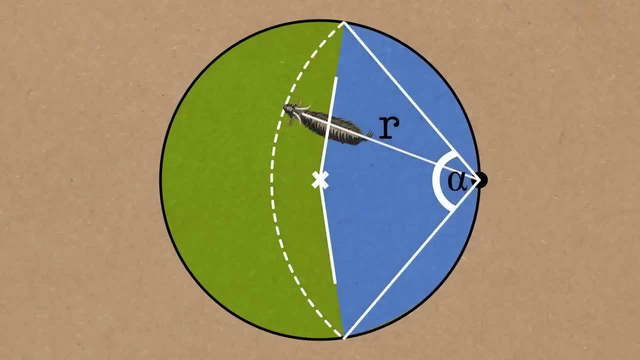 I can also work out if I start at the center here, a different circle, because I've missed off these bits here And so let's try and get those back. This is a fraction of a circle With a radius 1, and so we could talk about this angle and we could work out if I worked out that angle. 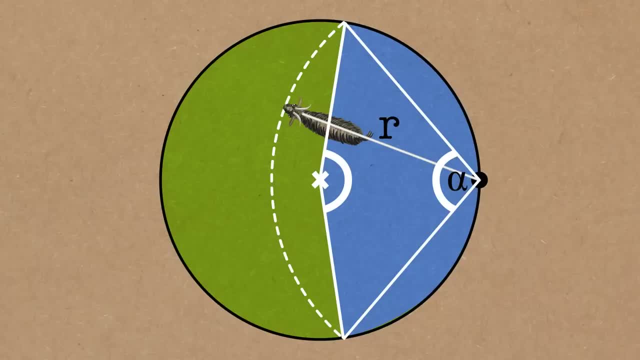 It's going to be related to alpha, so I'm not going to do all those calculations, But we can work out this fraction of a circle as well and then add it together and then we've got this area. But oh, no wait, hang on. 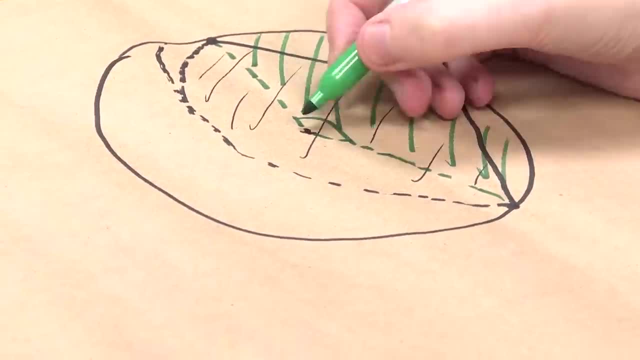 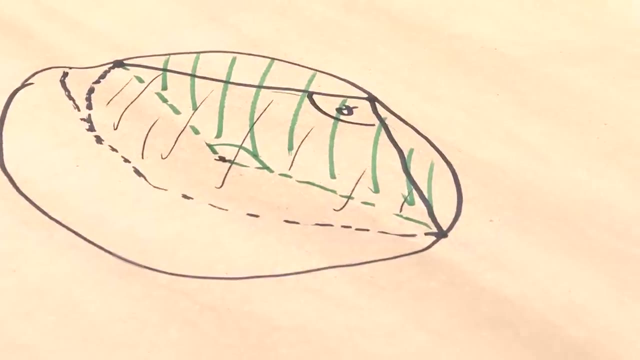 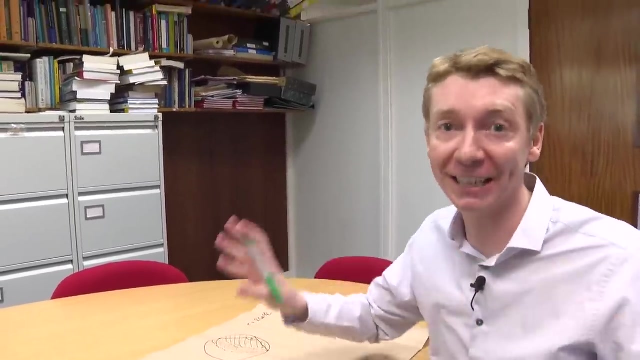 This diamond shape that I've got here. Can you see? it's overlapped. So I've got an overlap, kind of like two triangles, and it's all overlapping. You remove the overlap and then you've got the area the goat has eaten. I've not gone through the trig details because we would just be here looking at signs and causes for a long time. 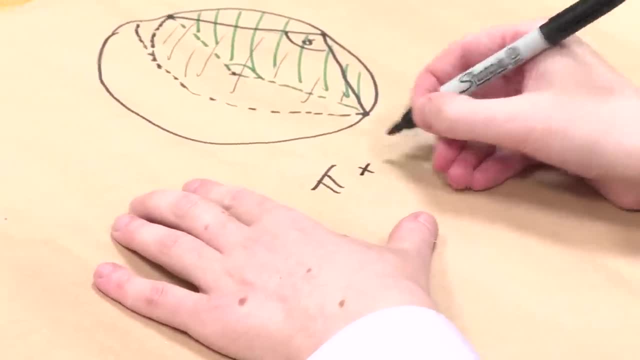 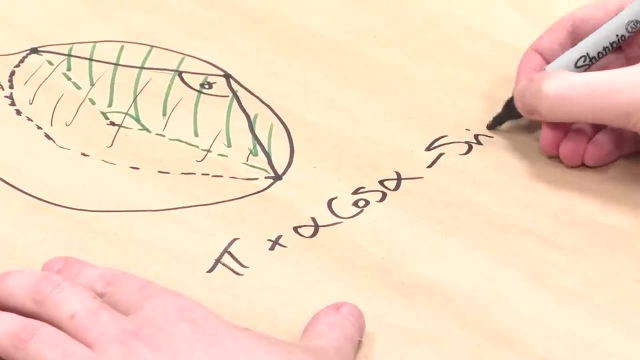 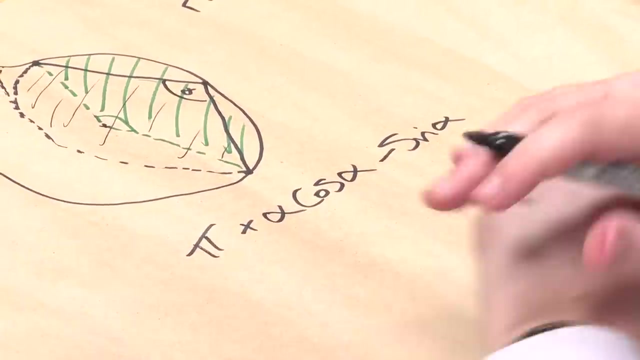 But this is what you would get: pi Plus alpha. so that's not angle cos of alpha Minus sine of alpha. That's the area that the goat is eating. Hopefully you can see why I didn't go through all the details, because it's actually quite a nasty. 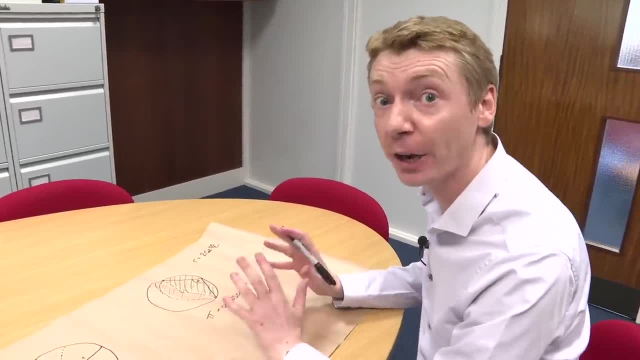 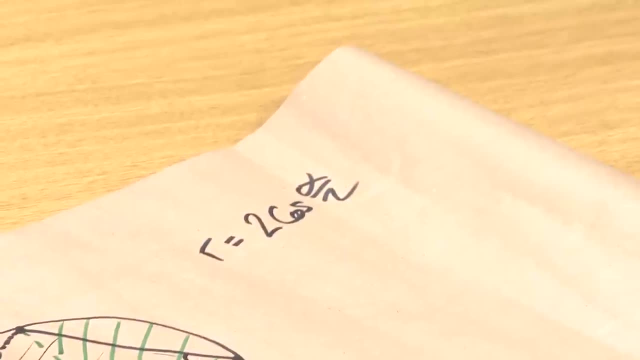 Calculation to do what we're going to get. then, if we solve this is we're going to find the angle alpha, and then that's okay Because I have a formula for the length of the rope there. That's where we come before we do one last step, and then we'll get that length of the rope. 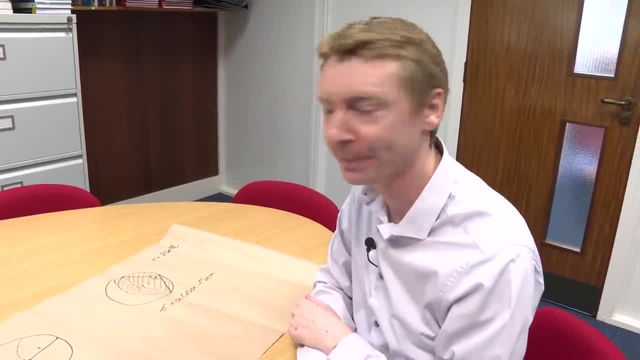 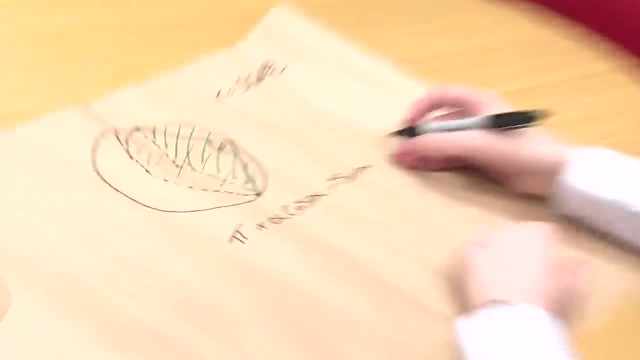 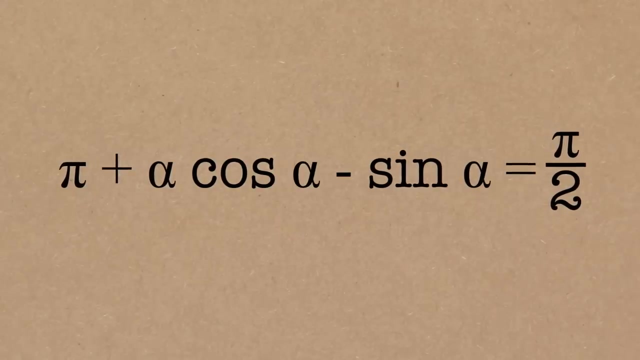 So it's actually calculating that angle. That's important for us for now, and we want this area that the goat is eating to be half the field, and Half the field is pi over 2, So we set this equal to pi over 2.. We're trying to solve this equation. It's not a particularly nice equation. 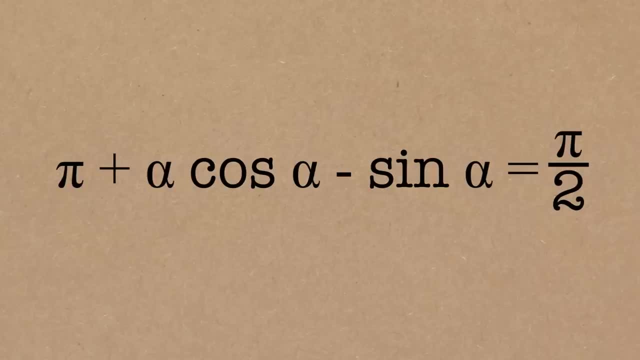 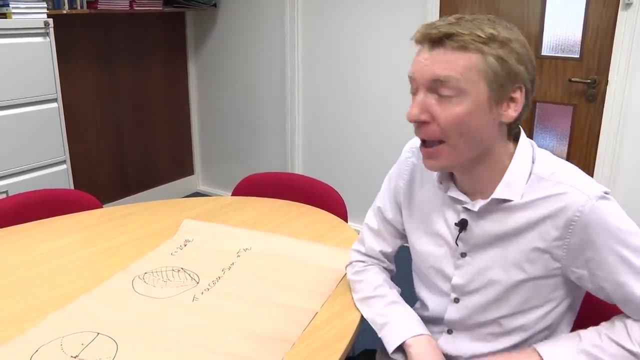 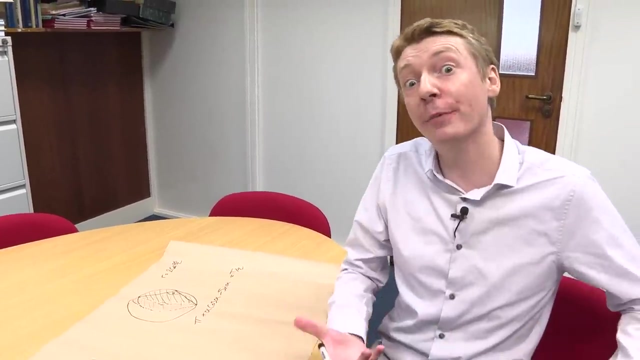 It's trig and in fact this is difficult to calculate because it's called a transcendental equation, So it sounds like a nice name but it's a difficult kind of equation to solve. a nice equation to solve is what we call a polynomial, and that's the kind of 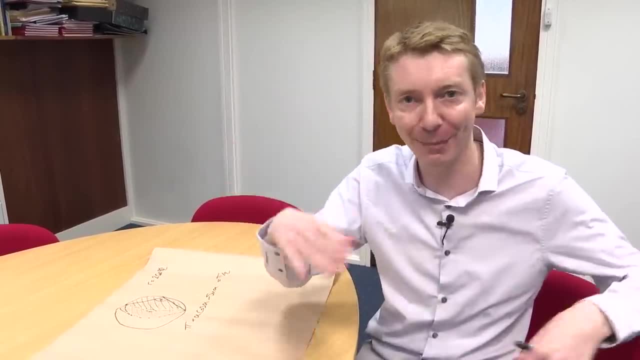 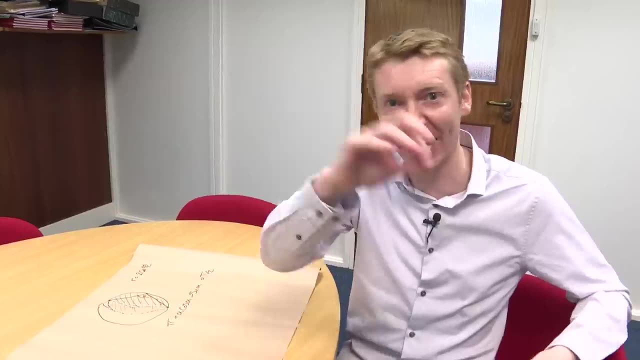 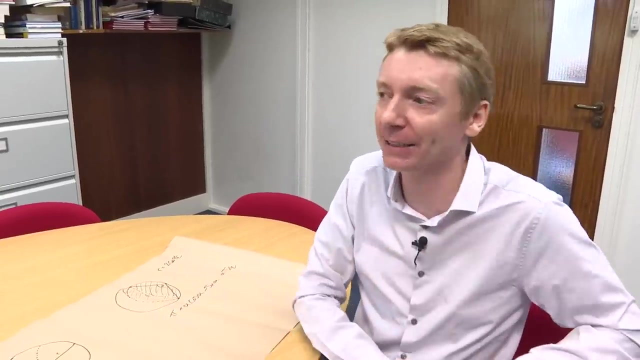 things you get where you have x squared Plus x minus 6, those kind of things. They're quite easy to solve and when you do, you get an exact answer at the end. So I can then say x is equal to. and I could write something down. It might have square roots and horrible things in it, but I can give you an exact answer. 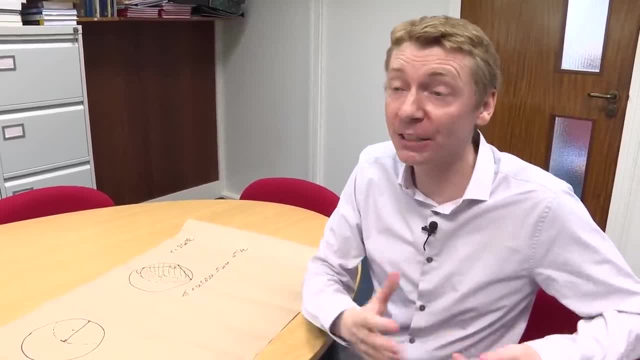 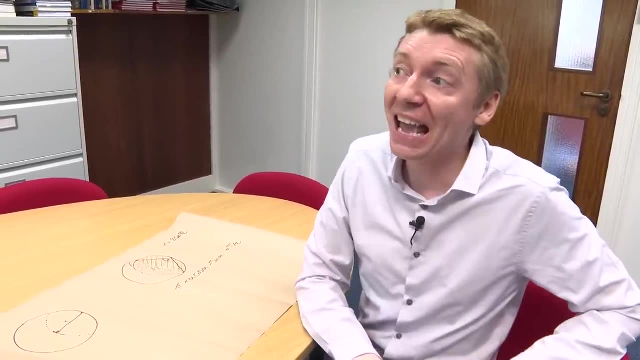 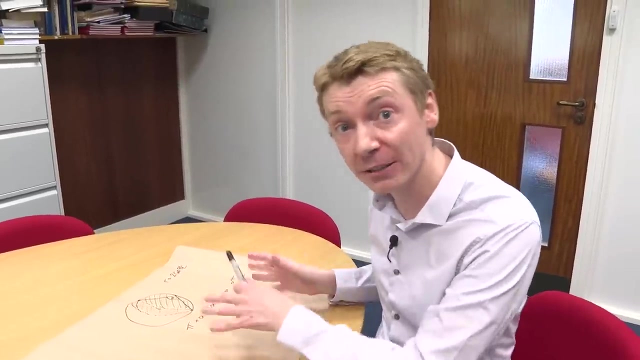 For a transcendental equation, I'm afraid there is no method for giving you an exact answer. the only way to solve it- and it's the angle we're trying to solve- is approximations is the only way to Solve it, and so that has been done, so we have an approximate answer for that angle. 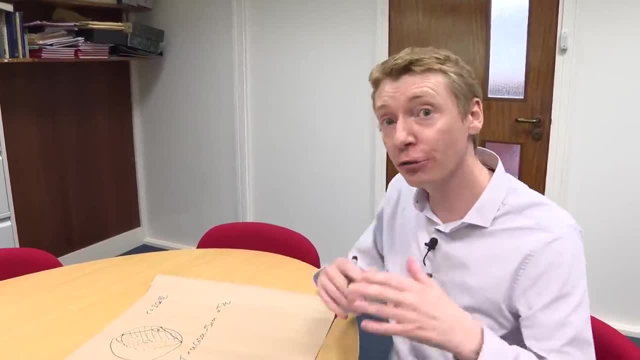 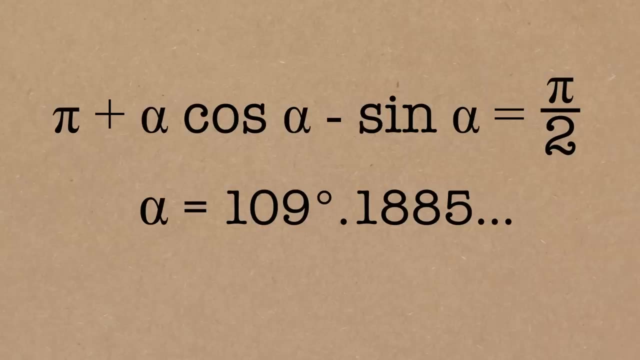 So we're getting closer and the approximate answer is it's about 109 degrees plus some decimals. So 109 degrees, point one, eight, eight, five, something, something, something. And we're not quite finished. the goat problem, because I want to know the length of the rope. and then really, the last step is: 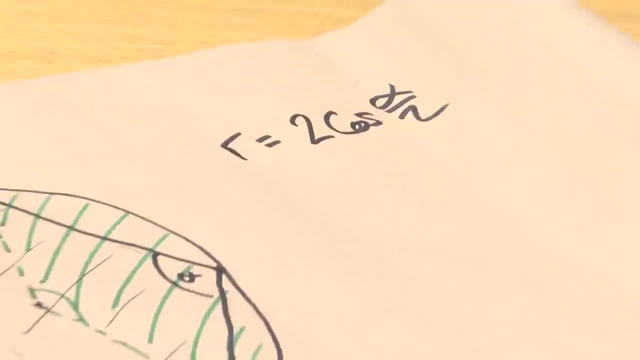 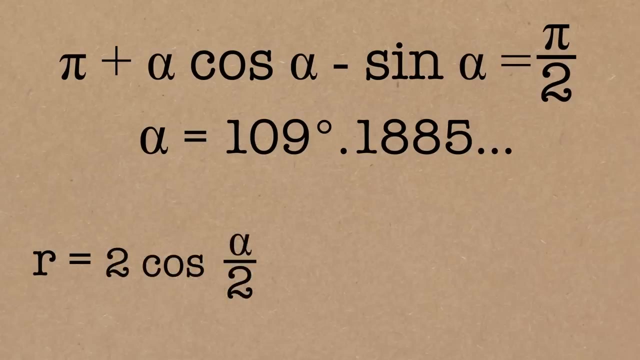 the easy step, Yes, the easy bit of trig. so showed us that the length of the rope should be two cos alpha over two. And that's going to be- and again, it's only an approximate answer, but it is this answer. one point one. five, eight, seven, two, eight. 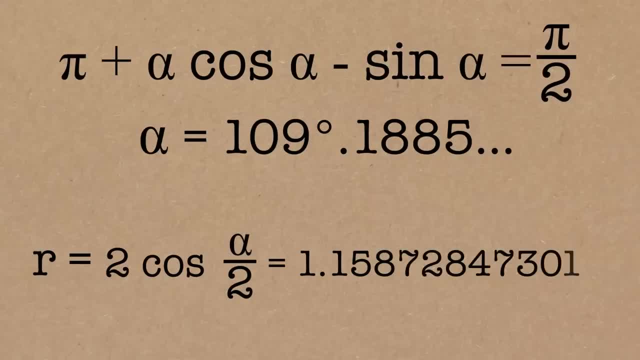 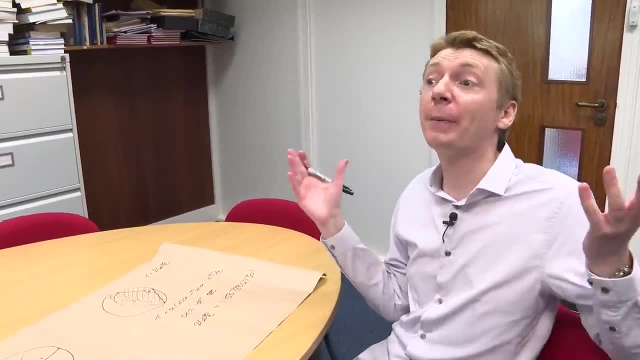 four, seven, three, oh one, dot dot dot. so just longer than the radius of the field. So it is, yes, a little bit longer than the radius of the field. I would have expected, if you asked me to guess, I would have gone Root two, square root of two, something like that. That's what the answer I expected it to be. 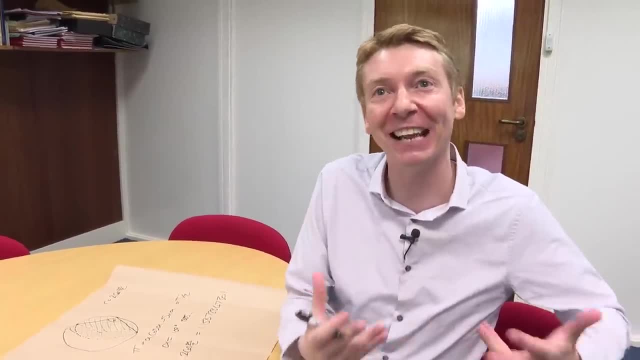 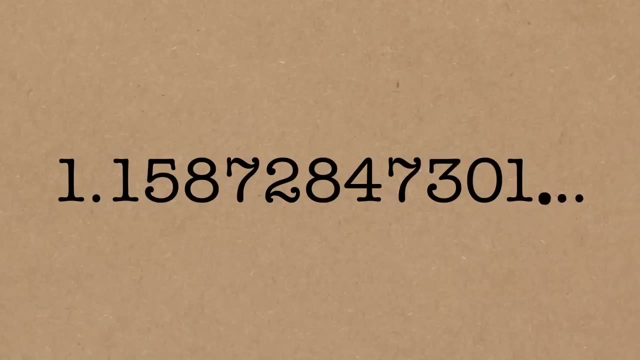 I think that's where some people get frustrated with this, because they want it to be an answer Like that, but it's not what we've got and there is well, until recently, there is no exact answer. It's that dot dot dot. that shows you it's not exact, It's a decimal. goes on forever. 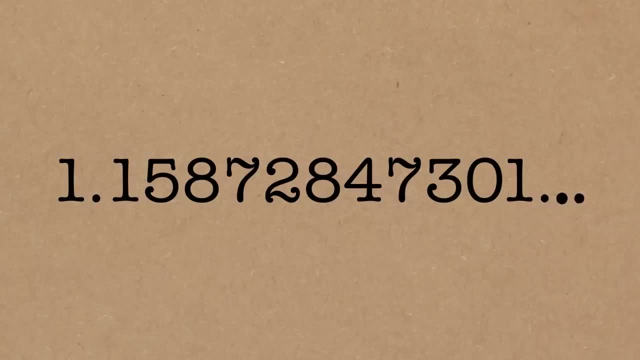 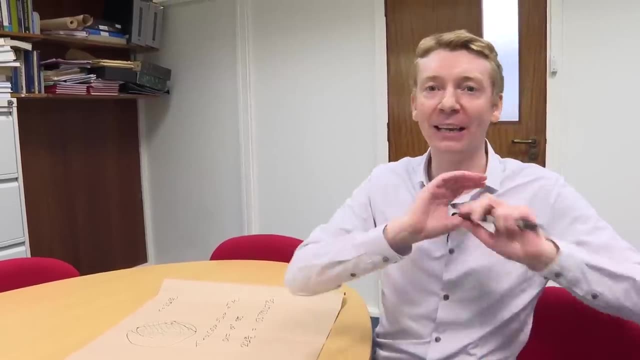 And yes, I mean we've got an equal sign, but equal dot dot dot. we can make this more accurate. You know you can make better approximations, But I could never tell you like an exact answer, like a little equation or a little formula Telling you what the length of this rope is. 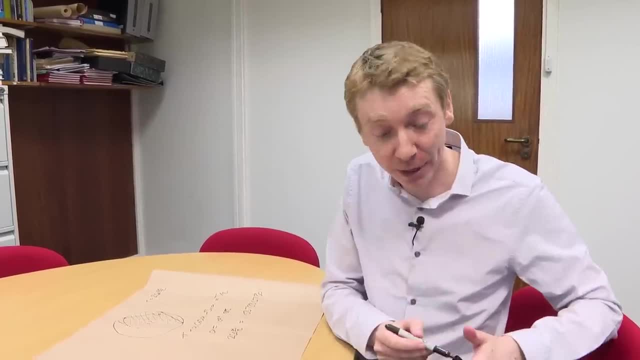 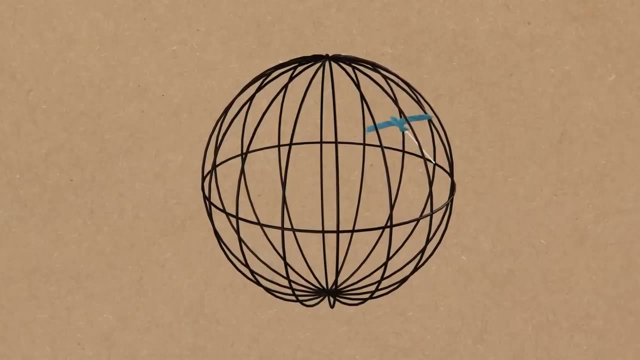 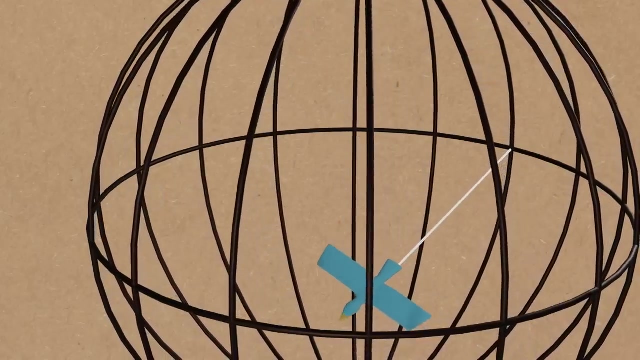 What's surprising About that problem- why it's surprisingly hard- is because the three-dimensional version of it is easier. The three-dimensional version is a bird in a cage. Imagine having a spherical cage of radius one, and you've got a bird tied with a thread and in that bird can then fly. 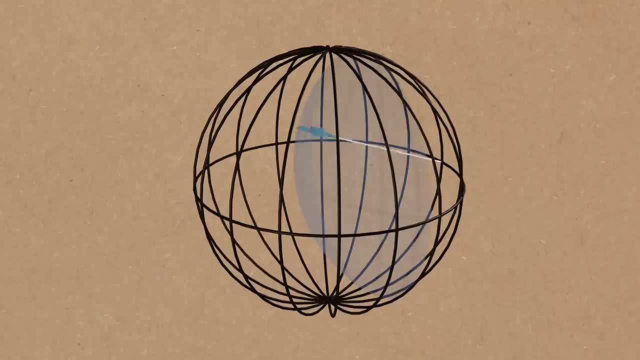 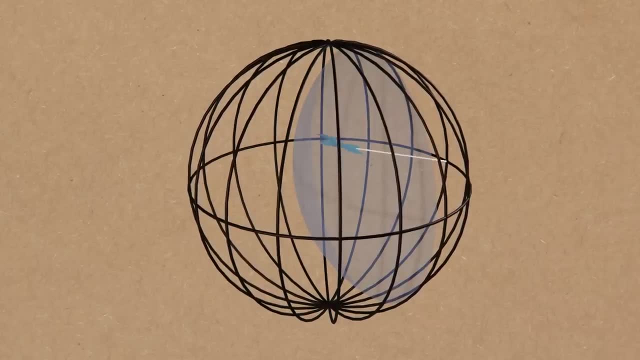 Wherever it's allowed to fly, limited by that thread, so it can fly around. What does the length of the thread need to be to be half the volume of the sphere? That should be a harder question. It turns out to be easy. Um yeah, you can actually solve it. Here's the answer. 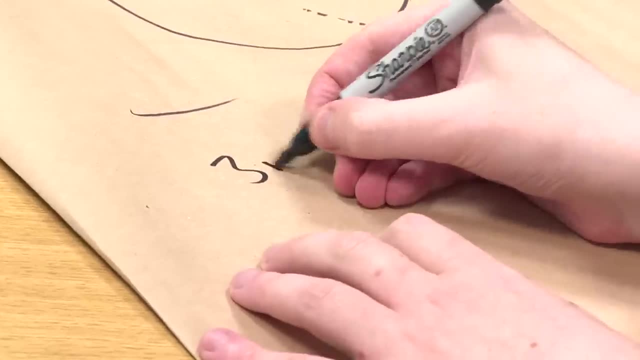 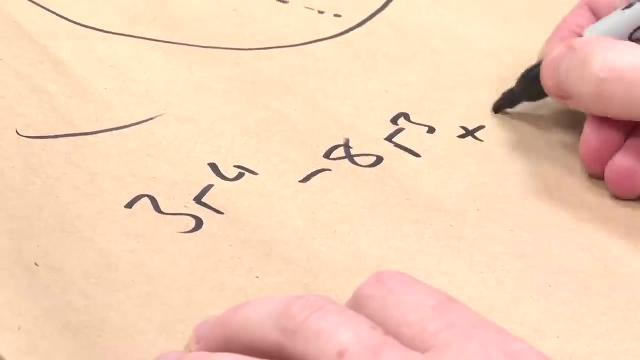 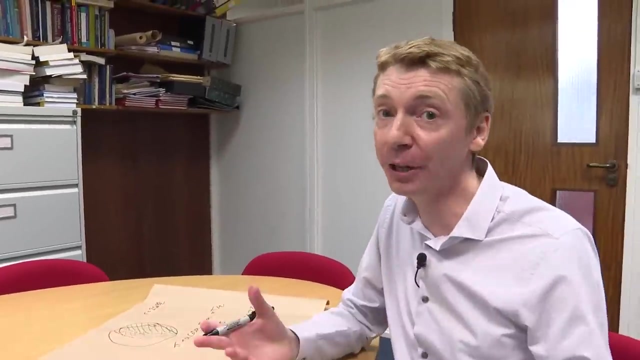 The equation you get to solve is Something like this: it's three R to power 4 Minus eight R, cubed Plus eight equals 0.. I mean, it's a traditional mathematical equation. It's a polynomial, and if it's a polynomial That will have an exact answer. it might have square roots in it. 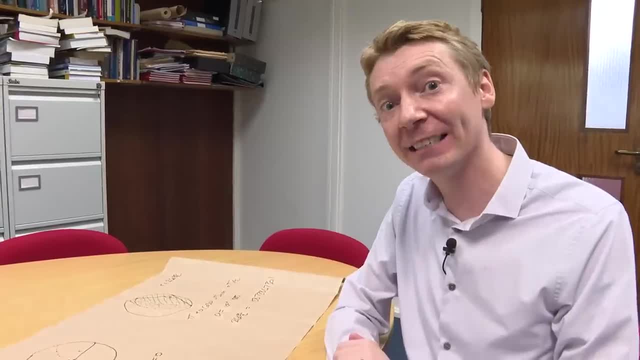 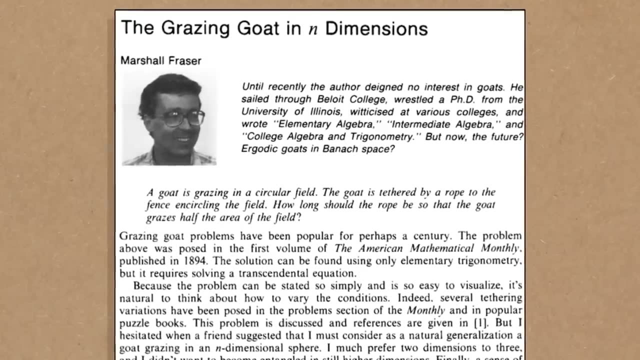 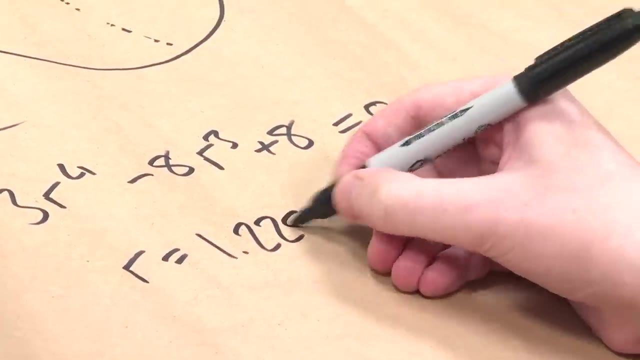 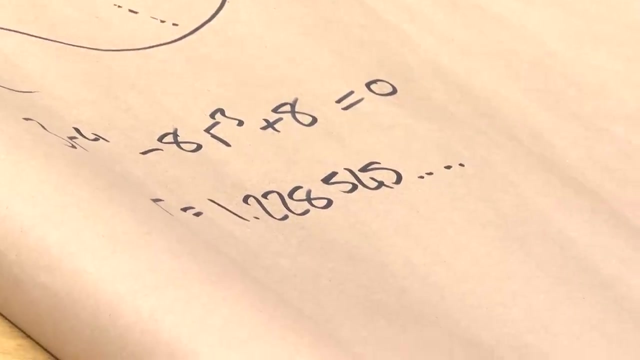 It might look a bit nasty have an exact answer. In fact, when this was solved, Marshall Frazier was a mathematician who solved this and he did give an approximation for this answer. His approximation was: that thread was 1.228545 and then something, something, something. So he did originally give an approximation. 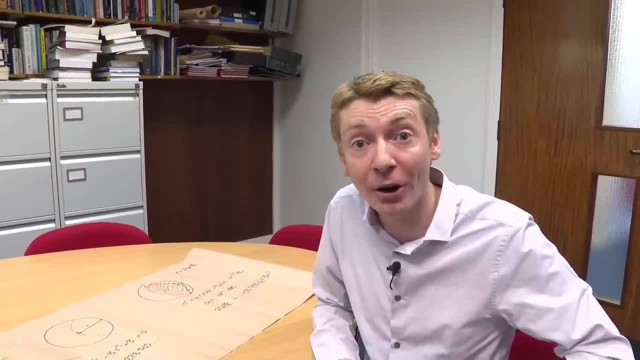 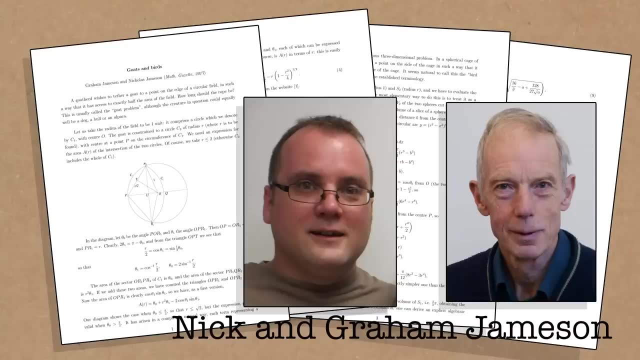 but a few years ago an exact answer was given And this is kind of nice for me. it was a couple of friends of mine who did it, so this is nice. I get to give them a shout out. This is Nick, and. 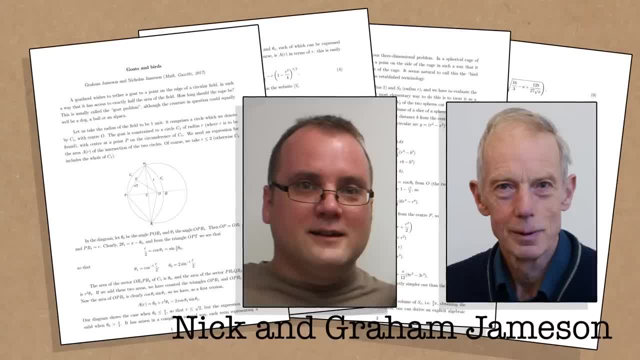 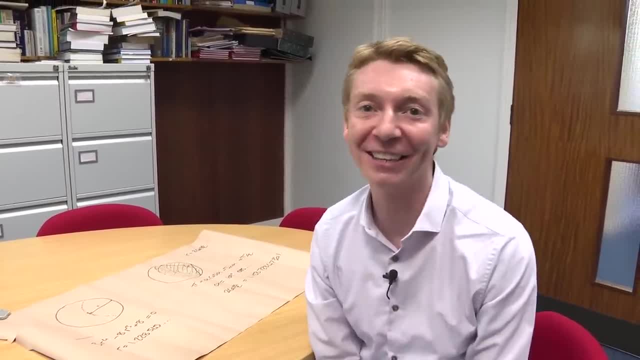 Graham Jameson. Actually, Graham was my lecturer at university and Nick is my friend for other reasons. So hey, hi, hey guys, This is really nice And they actually worked out the exact answer for the bird version of the goat problem. and it's this monster. All right, you ready, And it is a monster. 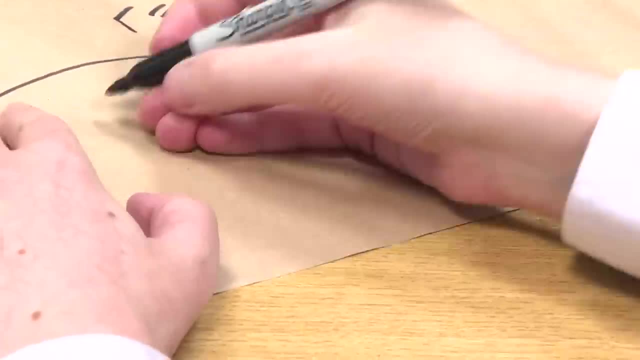 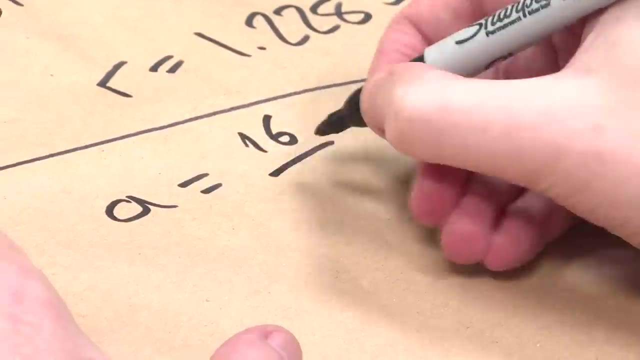 so are you ready? I'm ready. My friends actually broke it down into two parts because it's such a difficult thing to write down. They defined something called A, and this is a horrible thing as well. So A is 16 over 9 plus 4 over 3, and inside a couple of brackets we've got 4 plus square root of 8. 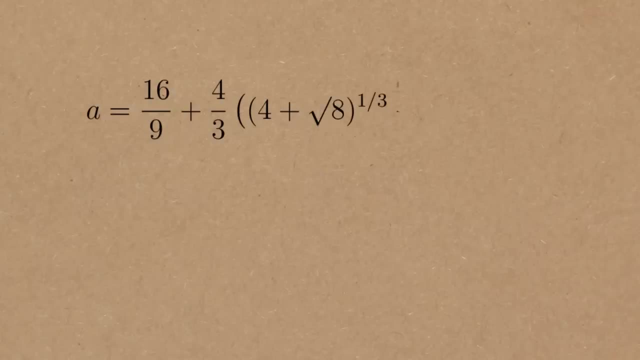 cubed rooted and then we add on another bracket here which is going to be 4 minus square root of 8 in a bracket, and we're going to cube root that as well, and then that's just halfway there, because then the length of the rope thread for the bird was going to be. 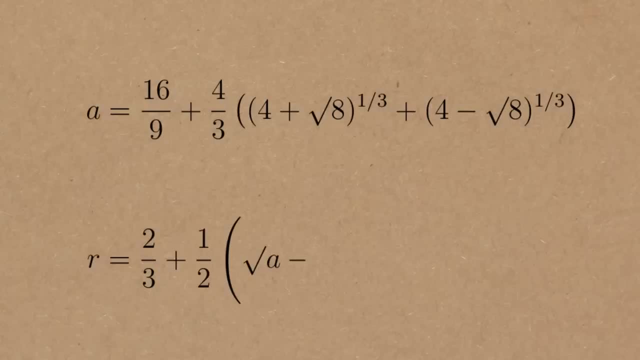 2 thirds plus a half of square root of A- that's where that A comes from- in minus. and then we've got another horrible thing: another square root of 16 thirds minus a wow, plus 128 over 27, and a square root of a down there as well. Whoa, It's ridiculous, isn't it? 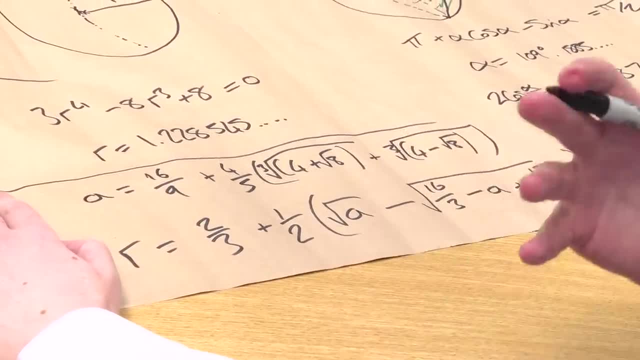 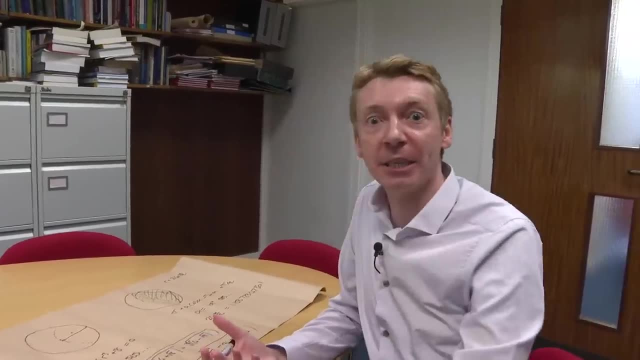 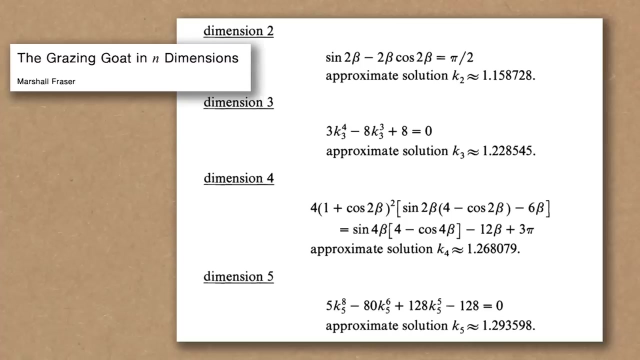 It's outrageous, but it is an actual, exact answer to this problem. So I could write that down as a decimal number. You could write that down as a decimal number. but I mean, that's what Marshall Fraser did. He didn't want to calculate that outrageous expression, so he said: well, 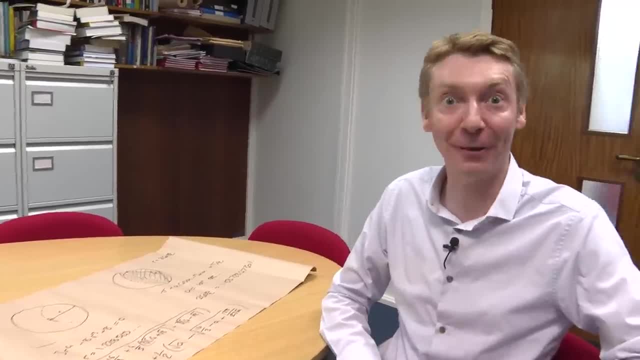 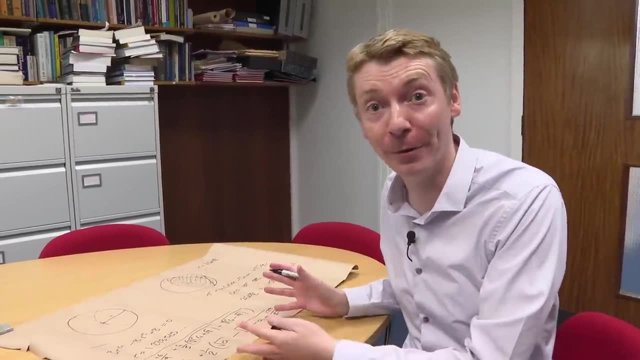 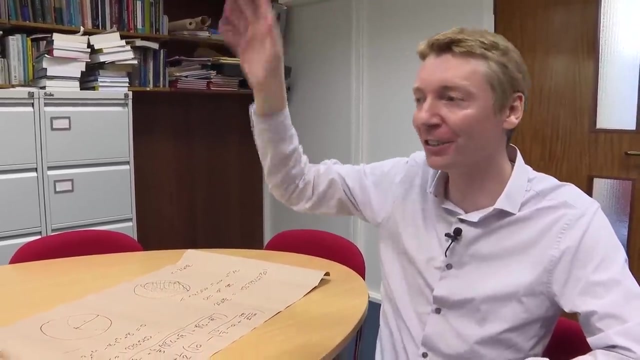 I'll just approximate it and maybe that's kind of more useful in some situations. but in this case this is a solvable problem. Actually, in higher dimensions it gets easier If you keep going up into the dimensions: four dimensions, five dimensions, so on the GOAT problem. 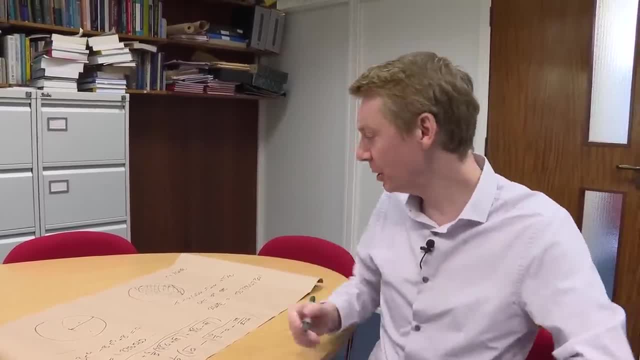 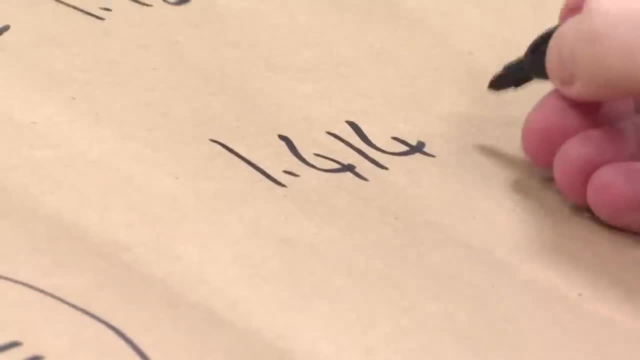 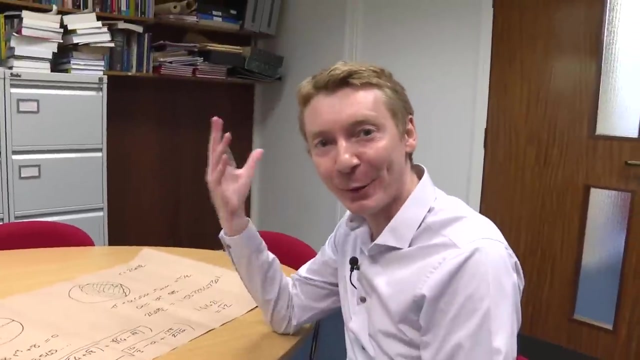 the length of the rope starts to tend to an answer, and it tends to 1.41421 dot dot, always the square root of two. It's. it actually tends to the square root of two. so it actually gets easier somehow as you go into higher and higher dimensions. and I would have expected the answer to be square root. 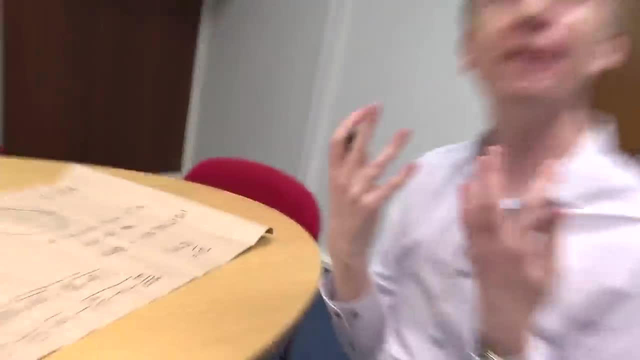 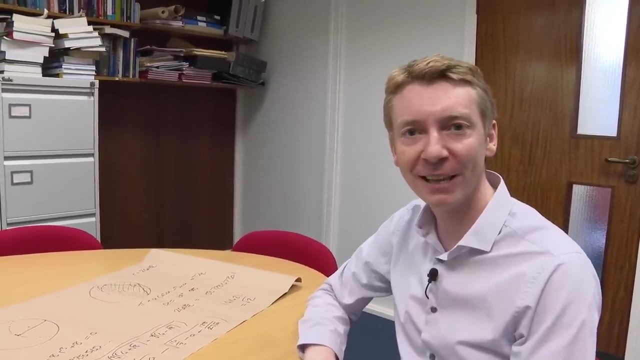 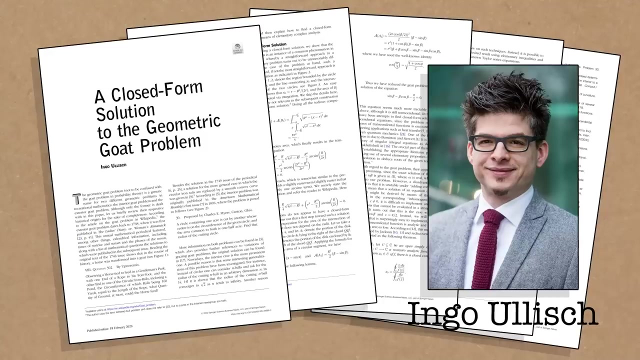 of two, just intuitively, that would be my guess, Like square root of two feels right to me. Maybe it feels right, but it's the two-dimensional one that caused all the problems. It's just really, really hard to solve. Well, until recently. we now have an exact answer. This has finally been. 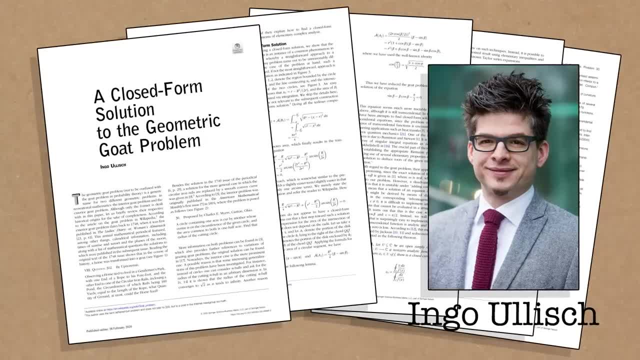 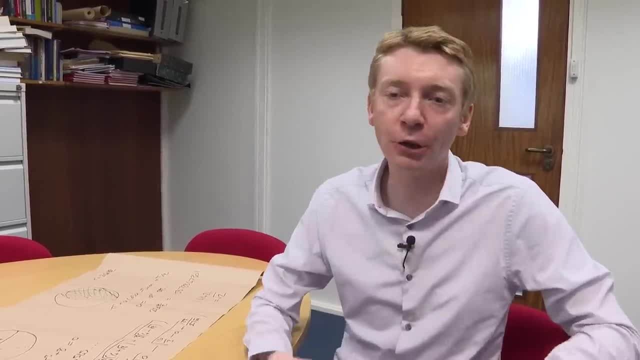 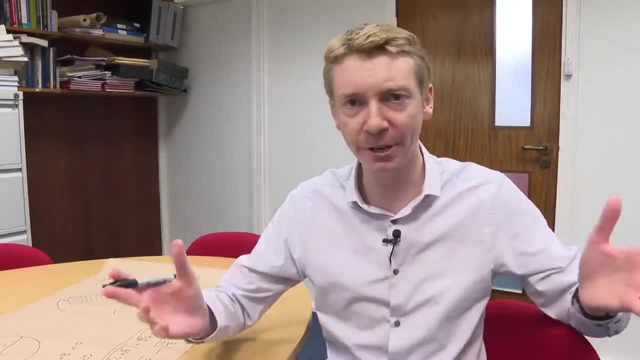 solved. It's been solved by a German mathematician called Ingo Ulrich, and to solve it he actually had to use some higher level maths. He used complex analysis. so he calculated that uses complex numbers and he calculated the areas using functions in complex numbers. They were like: 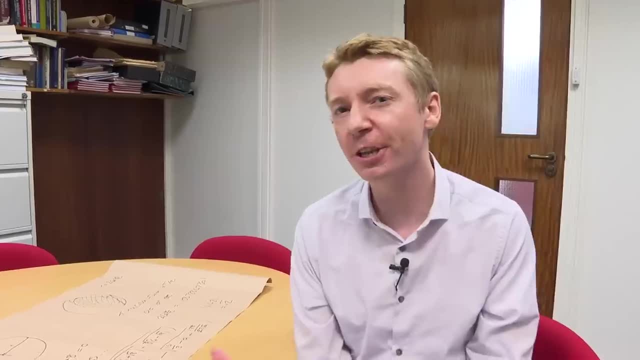 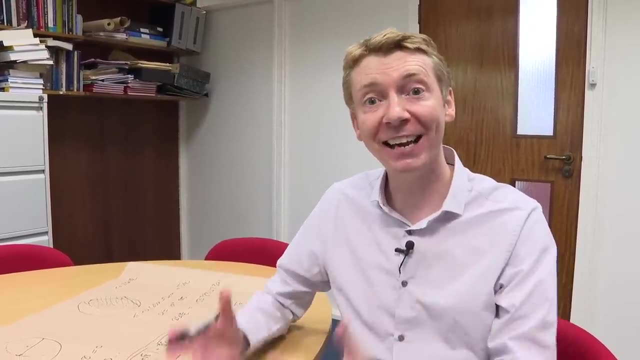 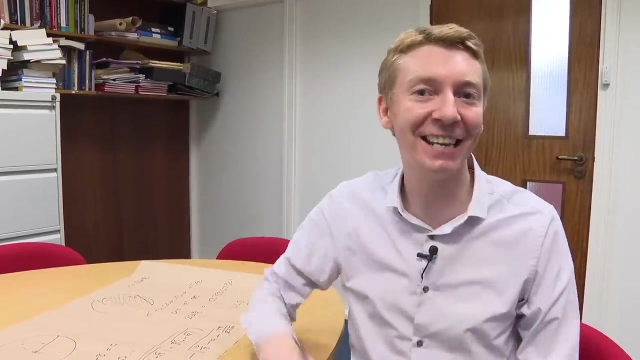 sine functions and cos functions, but now they're using complex numbers instead of the regular numbers, and worked out the area using this kind of maths and he found an exact answer. He found, he found the exact answer for that angle alpha. Once you've got that, then you can stick it into. 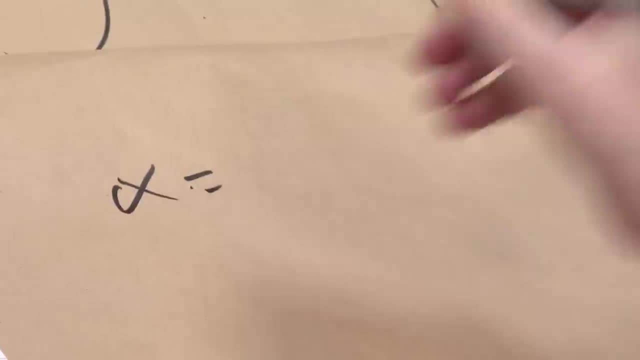 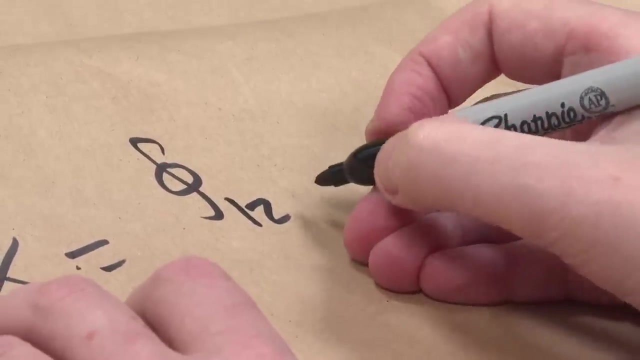 the formula we had before and it looks like this. So our angle alpha, that's what we wanted to know. It's an integral, it's a complex integral. That's what that symbol means and we're going to evaluate this when we do evaluate it at, z is a variable and all what we've got. 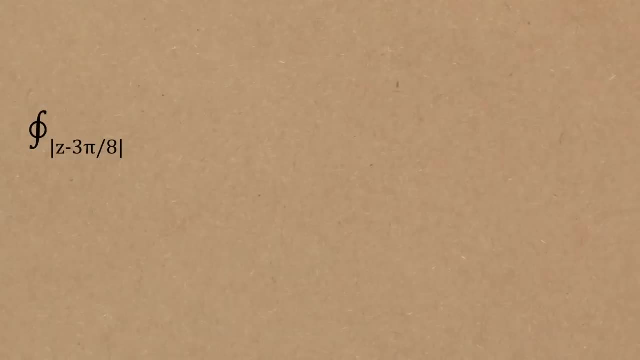 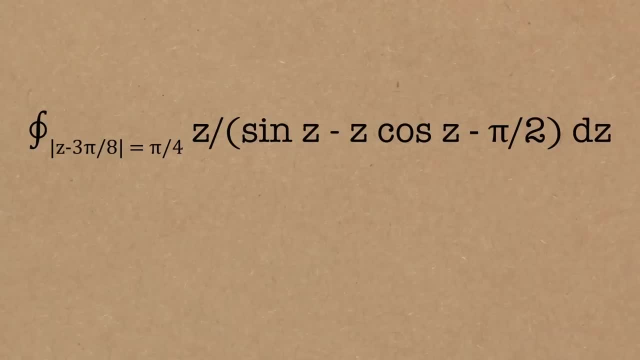 So we're going to integrate that- that's the dz, that's how you do that kind of thing- and we're dividing by another integral which is kind of similar. Whoa, It's outrageous, isn't it? But it's an exact answer. I mean for the first time. 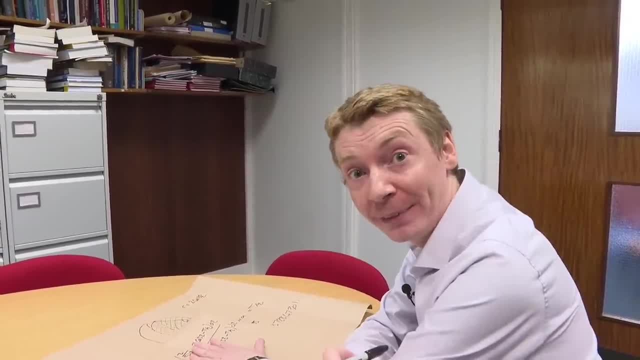 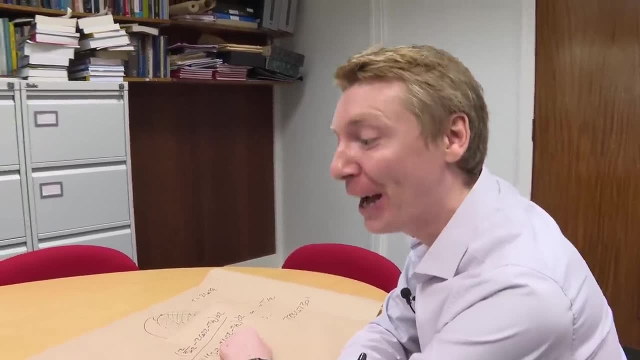 we've got alpha equals a formula, And how long's the rope? And how long's the rope? I mean, I'm just going to go back to our approximation, because it was easier to work out, which was what I said earlier, which was 1.158.. 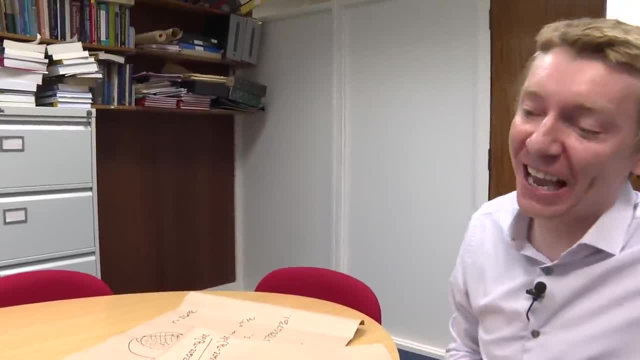 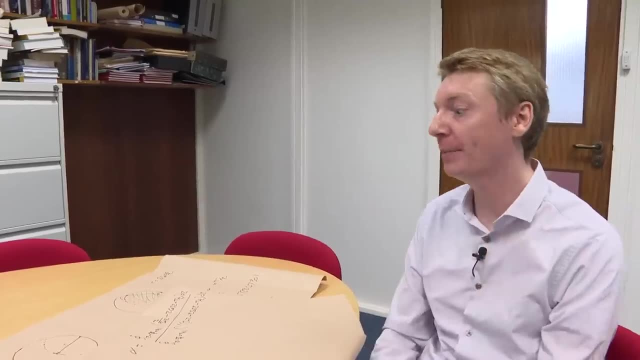 So it's pretty much the same. it's just: Oh, it is the same. it is the same, In fact. I will tell you this: it's really nice to have an exact answer. I mean a formula for the first time, Although this formula is hard to work out. 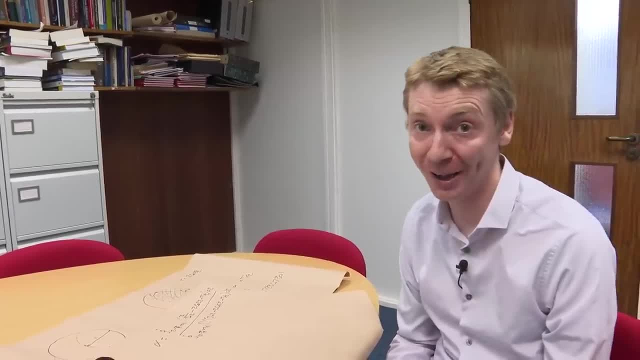 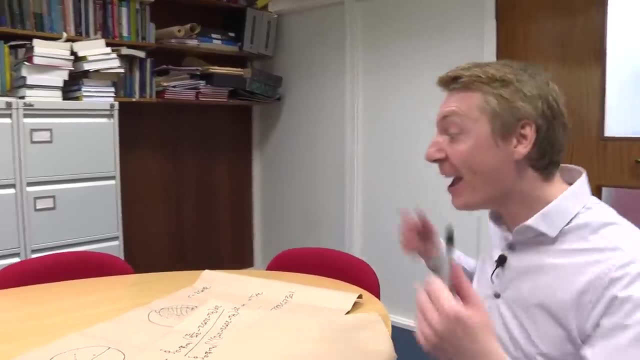 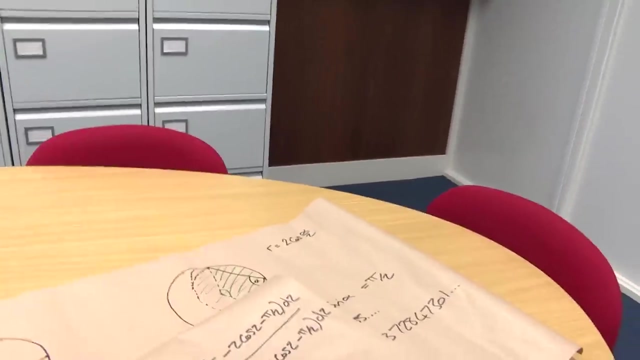 and if you wanted to work it out, you'd be better off approximating the values anyway. So it's still calculated by approximations. But hey, we've got the first formula for the angle alpha, So you would then put that into. You then take that alpha. 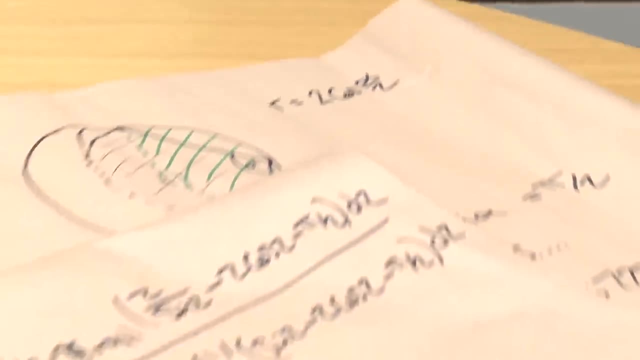 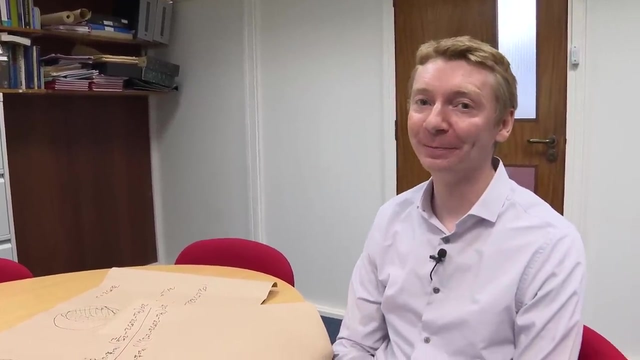 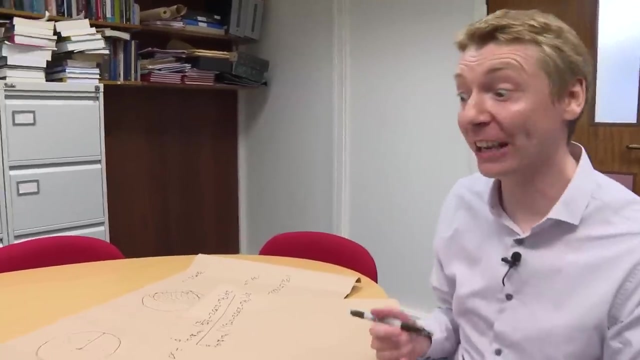 put it straight into the formula that we had with our trig: So the trig is still there as our final step And that's just going to change the length by like a billionth of a nanometer, sort of thing. Yeah, I have no idea. I have no idea Because I don't think it's actually been calculated. because it's hard. So we know the exact number, but no one would probably bother calculating. You couldn't put that into a wolfram alpha. I don't think we can. I Even wolfram alpha, I think, would struggle to calculate this answer. 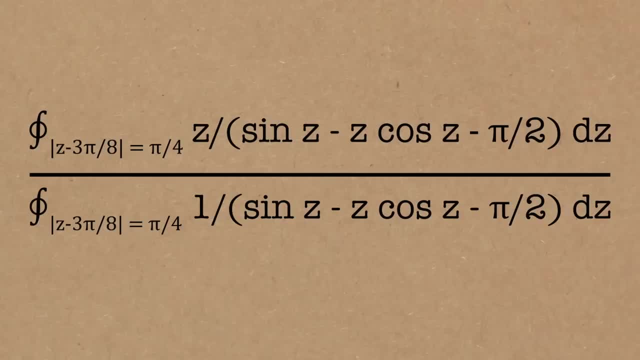 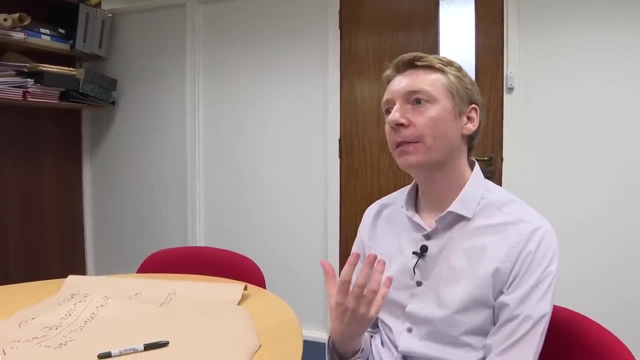 Why did this mathematician do this? Why did he spend his time? just because I mean I don't want to speak for him, but I can guess if you want. I mean it is an exercise in his methods in mathematics, It's practice. 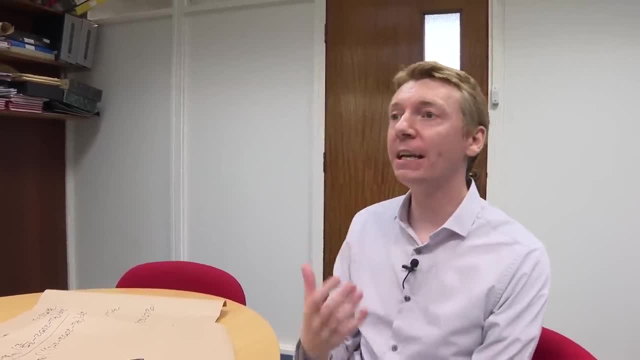 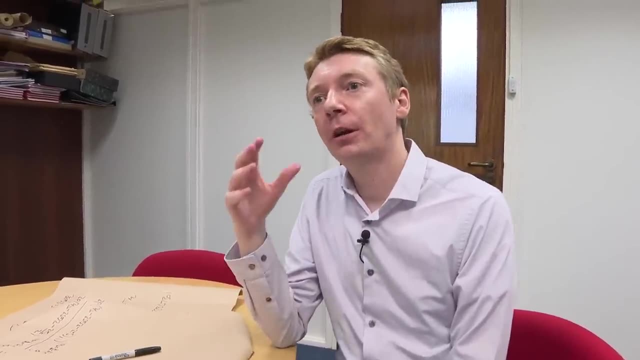 And then you know this is not an important problem, but it is a way to practice. you know your tools And then you can use that practice One day in the future for problems you do care about. Okay, here's a puzzle for you. 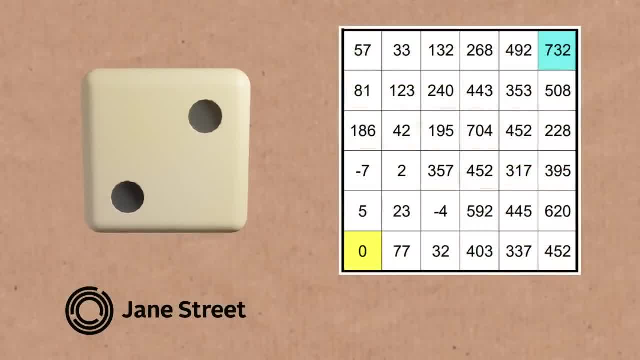 It involves rotating a die using the numbers on the face and moving it around this board. It's the latest brain bender from Jane Street, today's episode's sponsor, And to check out the details, have a look at their website. 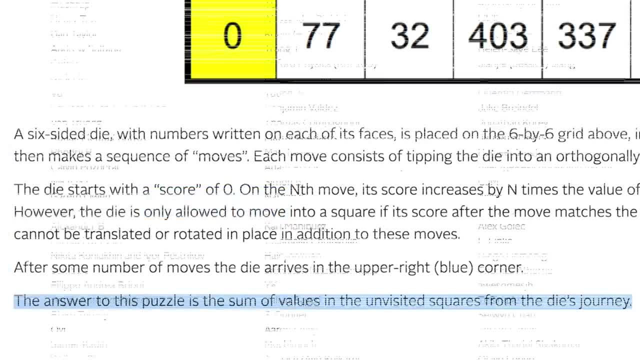 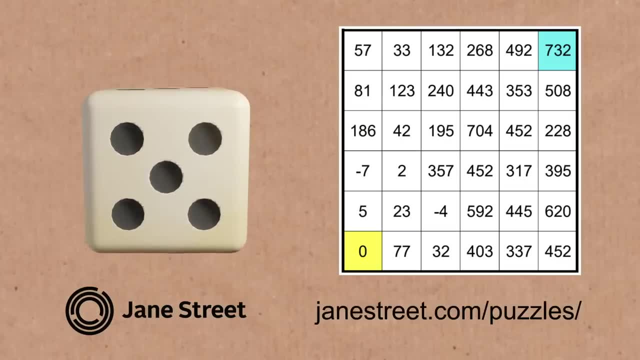 There's a nice clear explanation there, And you'll also find a wall of fame for people who have already cracked the puzzle. Maybe your name could be added. See the link on screen and in the video description. And while you're there, why not check out some of the latest jobs and opportunities?